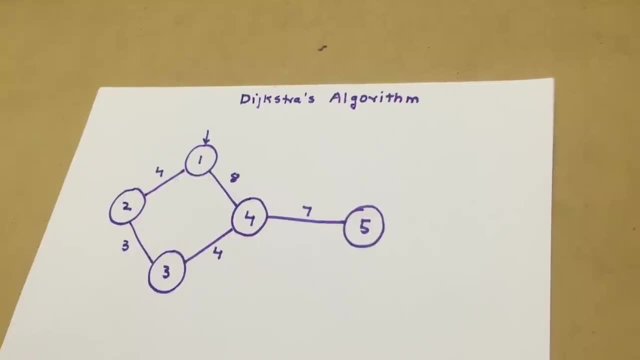 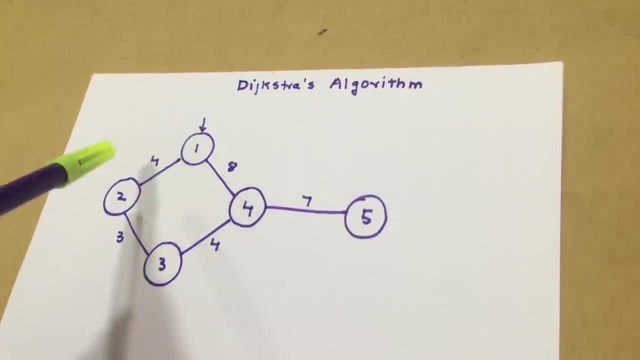 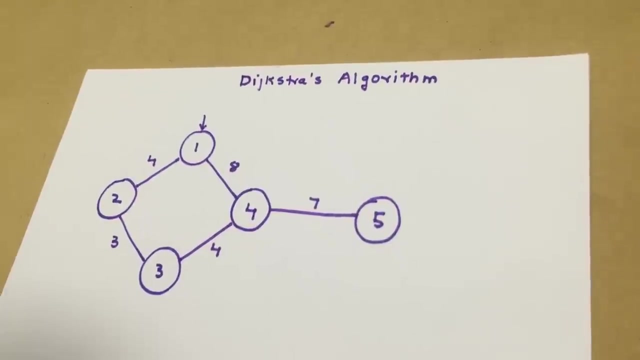 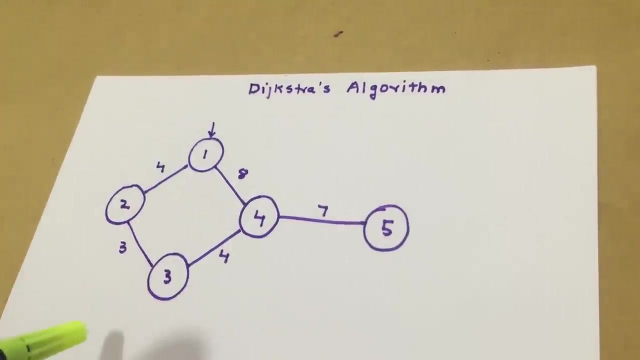 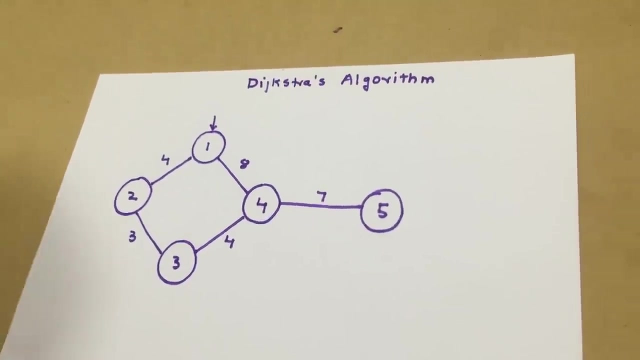 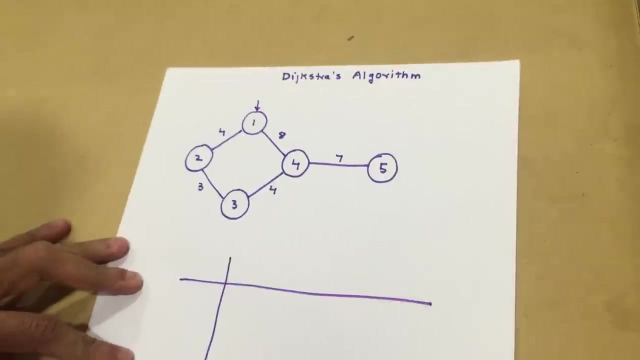 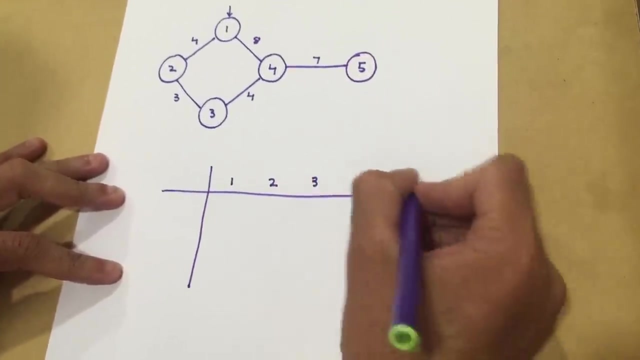 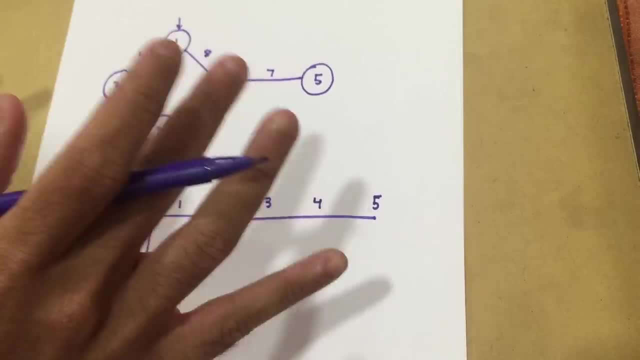 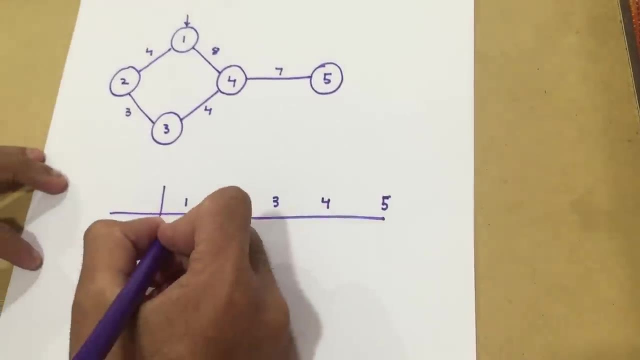 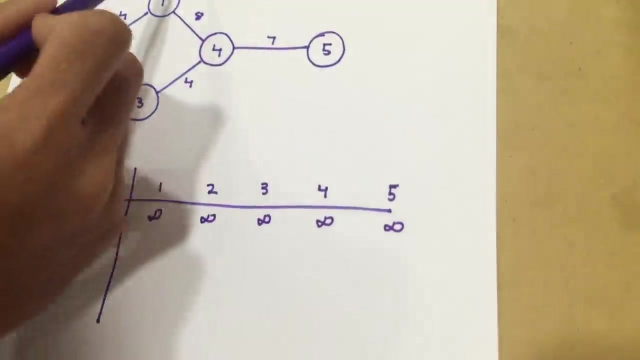 you are at one node which is not in any of this, which is not present in the network, so your distance from that node to any of the nodes is infinity, right? so initially all the distances are infinity. now suppose you want to start from the root node. so if I start, 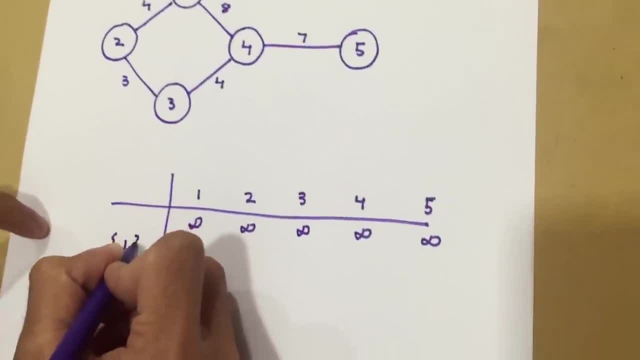 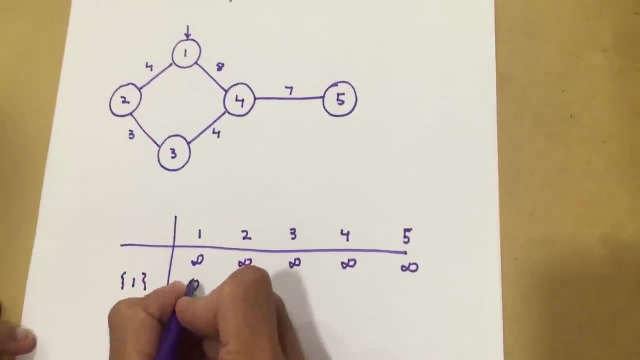 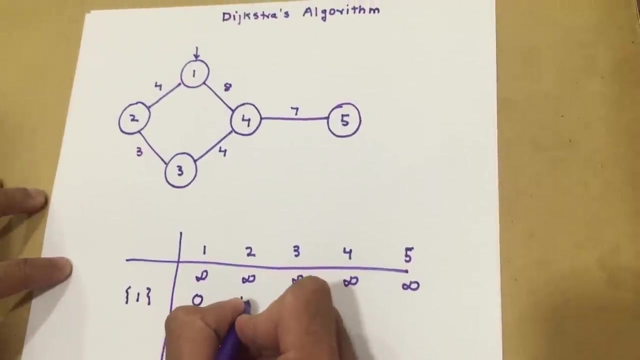 from the root node. initially I will start from one, which means I am present at one. so if I am at one, then my distance from one will be zero. from two, since one and two are connected, the distance from two will be four, since one and three are not connected. they 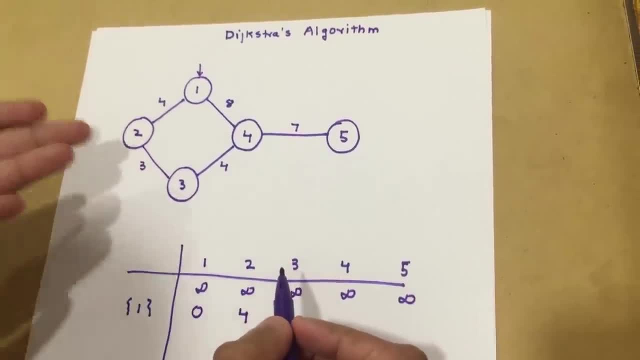 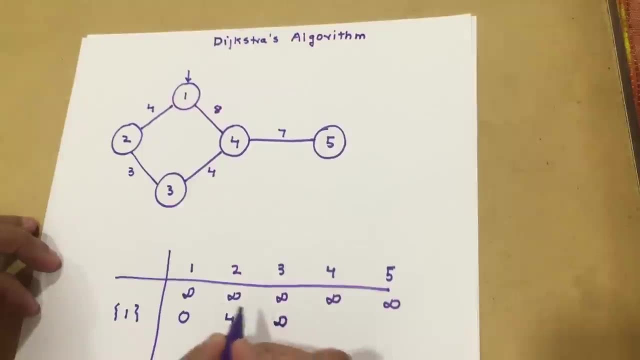 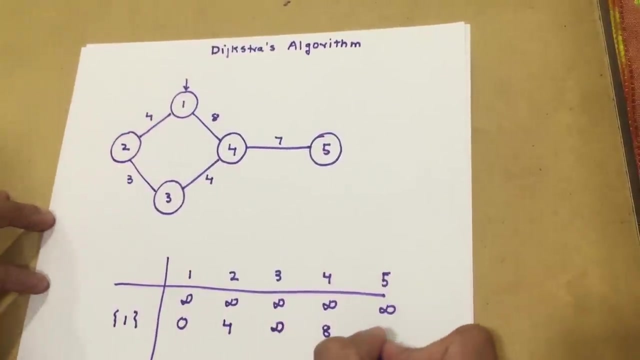 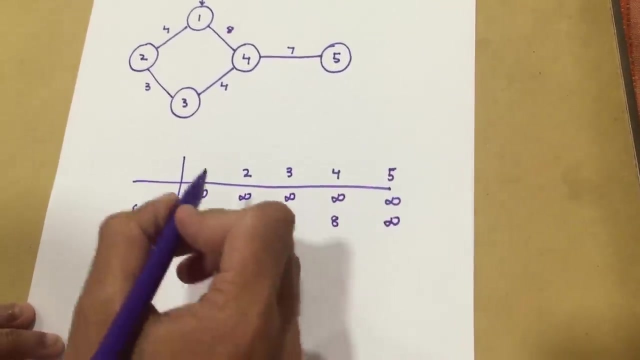 are not directly connected. so distance between, there is no distance between one and three, so we are going to name it infinity. four, now, one is directly connected to four, so the distance between one and four will be eight. five is one connected to five, no, so again, distance will be infinity. now what we do? we have this row, we see, which is the. 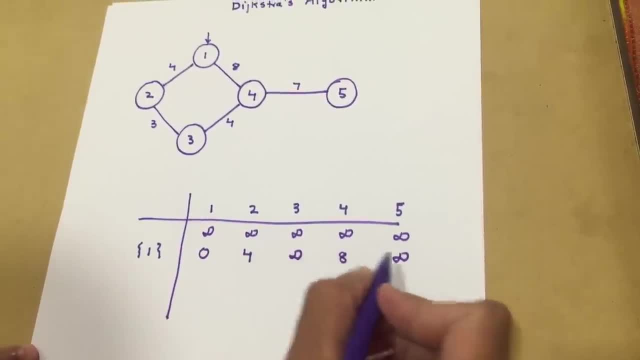 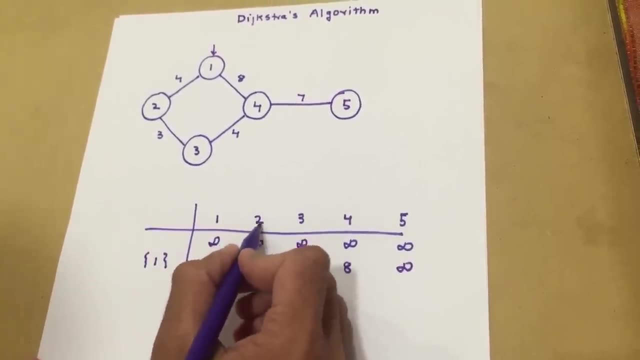 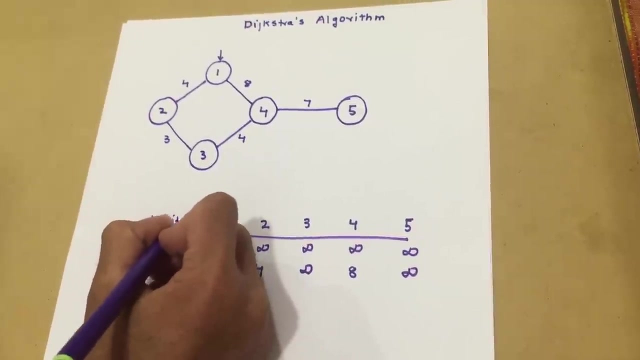 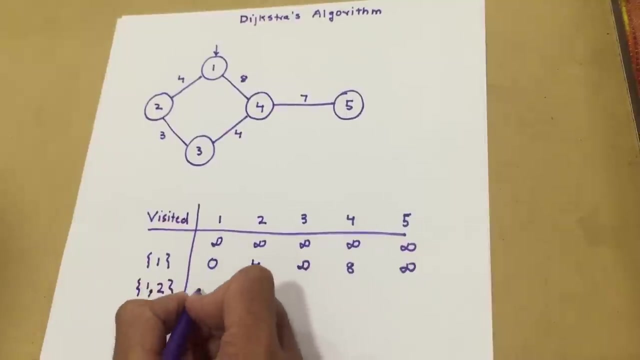 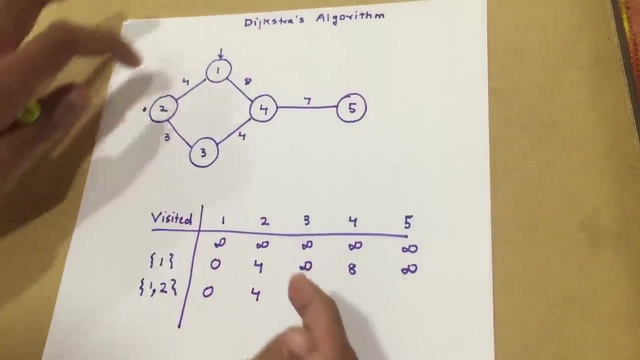 minimum distance here: zero, four, infinity, eight, infinity. the minimum distance here is four. right since we have already visited one, so next we are going to visit node two, since this has the minimum distance of four. so this is my visited column. so the next node I am at is two. so this will remain zero. this will remain four. now I am at two, so from two I 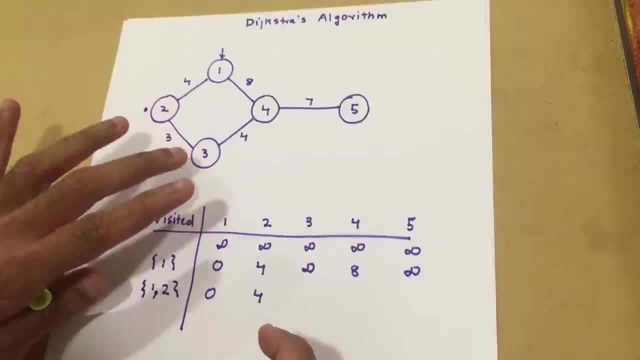 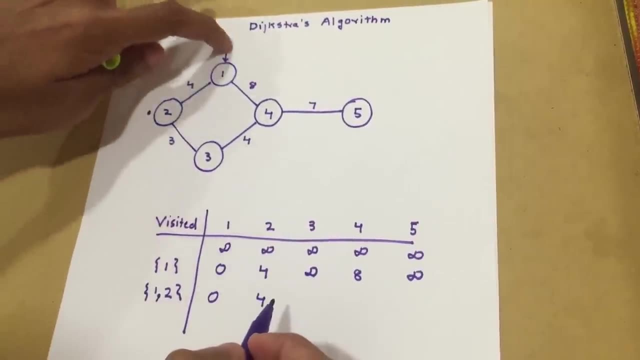 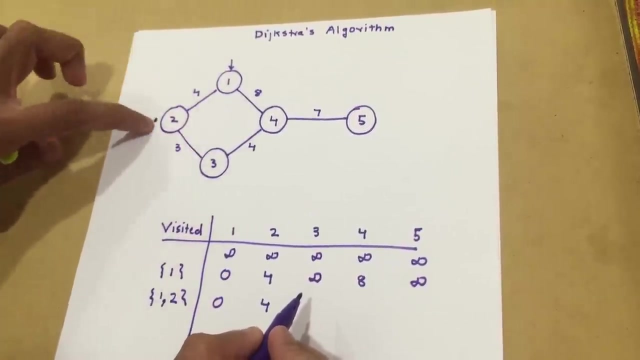 have one and three. since we have already visited one, we are going to only look at node three. so what is the distance of the node three? but since we started from our root node, we have to check from one. so what is the distance of three from one? four plus three, seven, right? 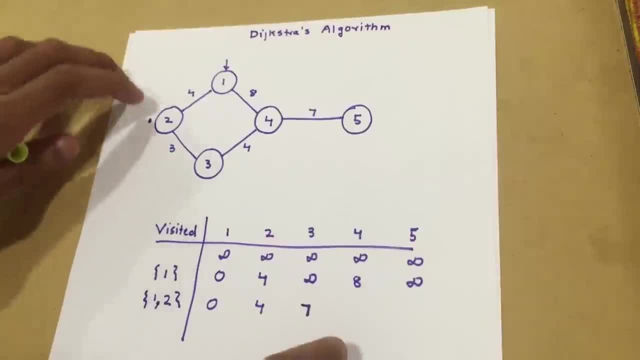 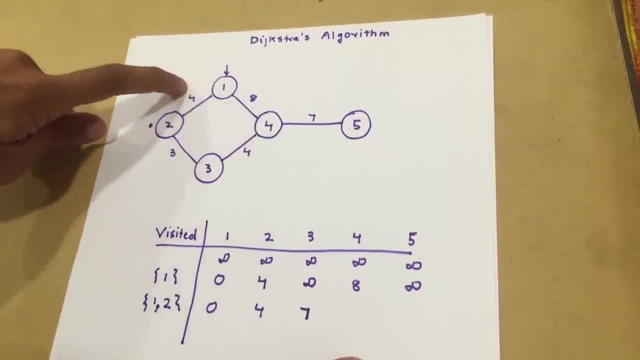 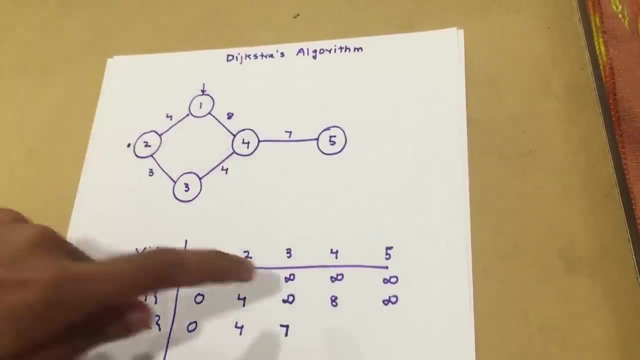 since this is infinity, we will change to seven, now four to see four. we will have to check this path right. so what will be the distance? four plus three plus four, that is what eleven. but earlier the distance from one to eight was already eight. one to four: the distance, 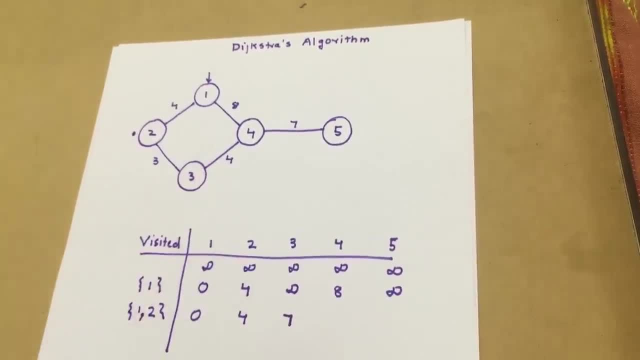 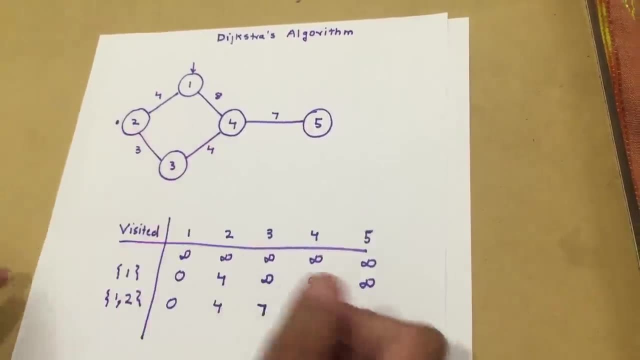 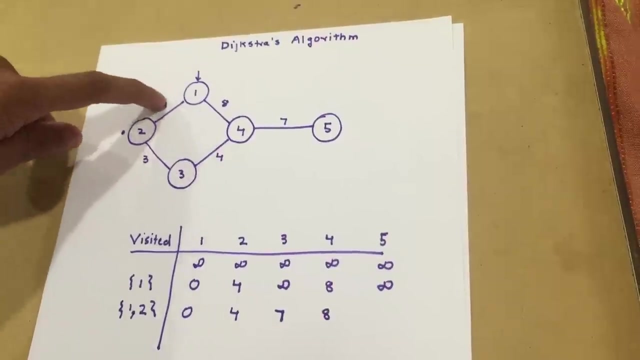 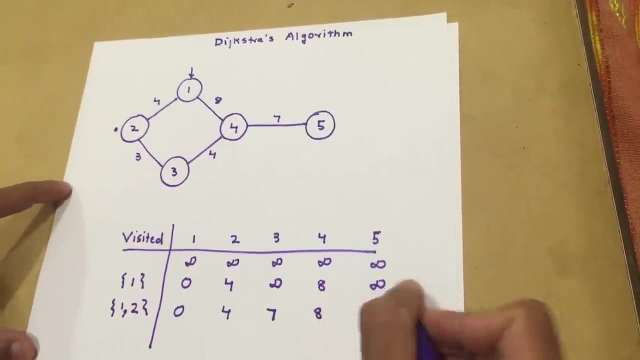 was eight and from here this path, if we take the distance, is coming to be eleven. so we have to choose the shortest path. so, even though it is coming eleven this way, we let it be eight, and for five, this distance will be what four plus three, seven plus four, eleven plus seven, eighteen, since it was infinity. 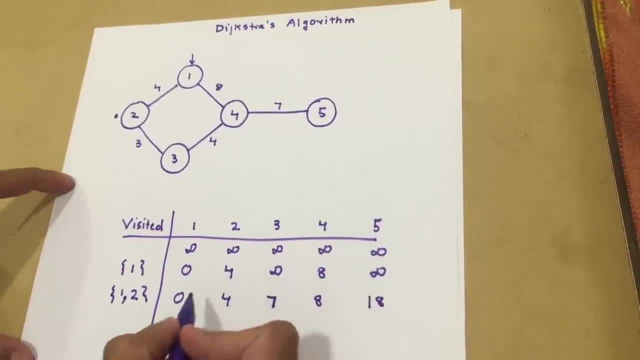 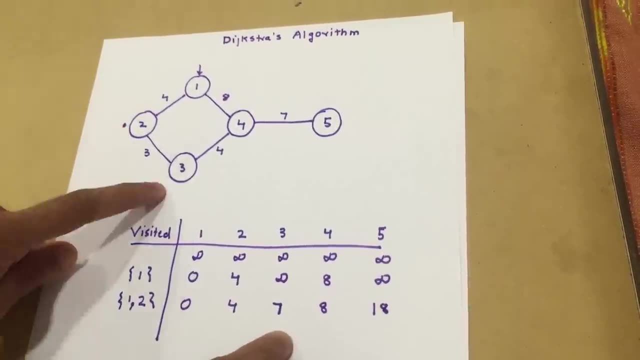 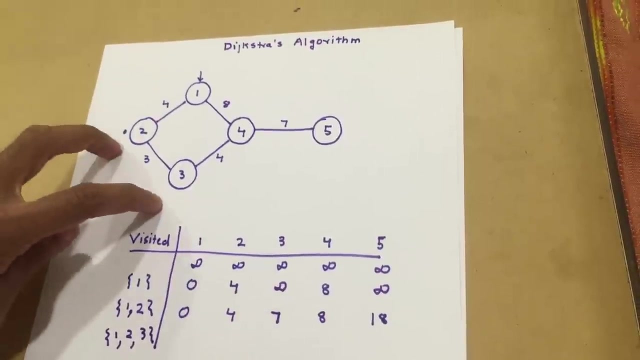 eighteen is lesser, I will put down eighteen. okay, so now I have visited one, two now, which is the smallest among seven, eight and eighteen, seven, right, so the next node we visit will be three, okay, three. three is connected to two and four. we have already visited two. 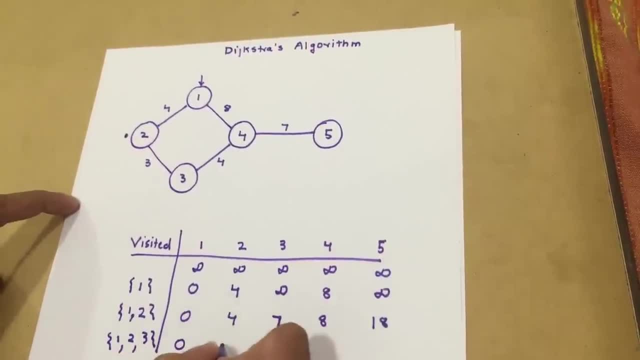 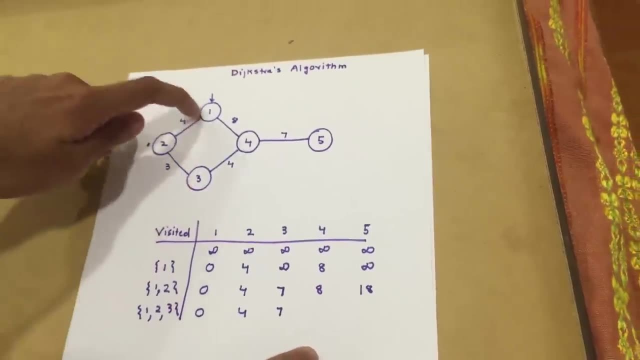 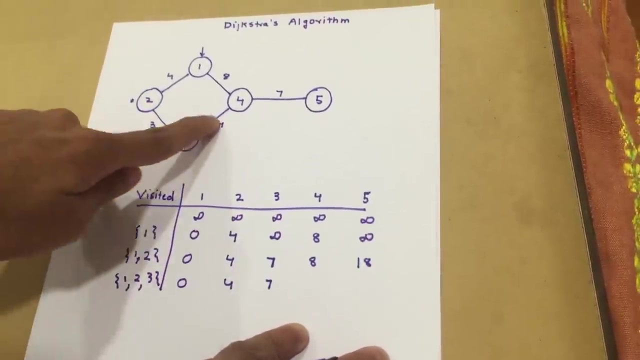 so that leaves us with four, so I will write this down as it is okay. so now, what is the distance? if we same way, if we go, if we travel all the way here to reach four, the distance again will be eleven. but from one to four, the distance will be eleven, and from one to 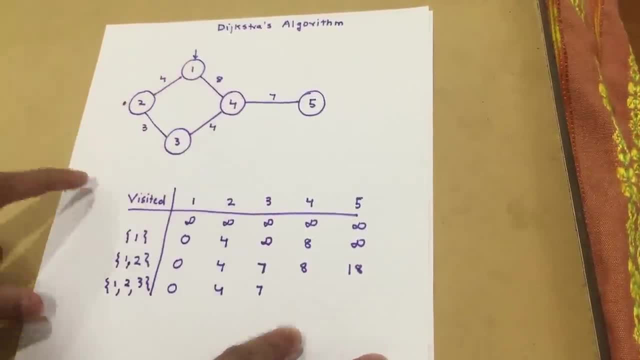 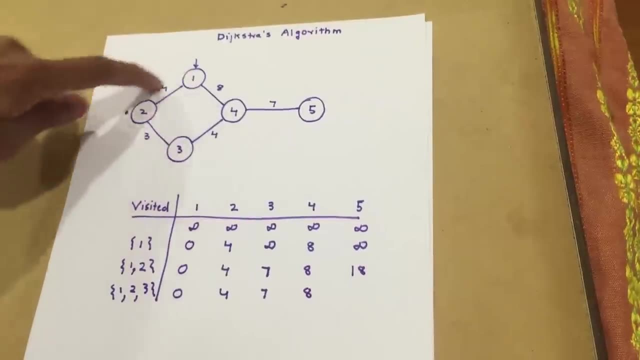 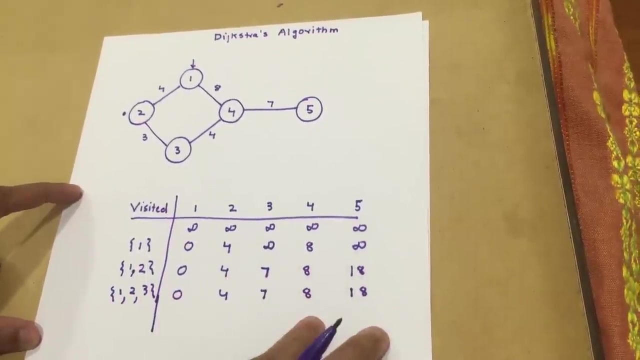 five, the distance is already eight, so we cannot change that distance. so this has to be eight. and for five again to travel through three, we have to take this path. so the distance remains the same: eighteen now, between eight and eighteen. eight is smaller, so next we are. 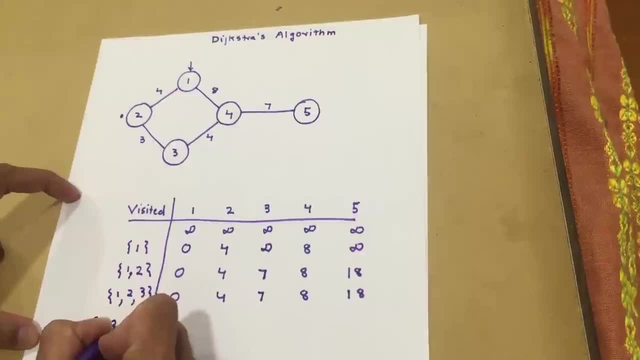 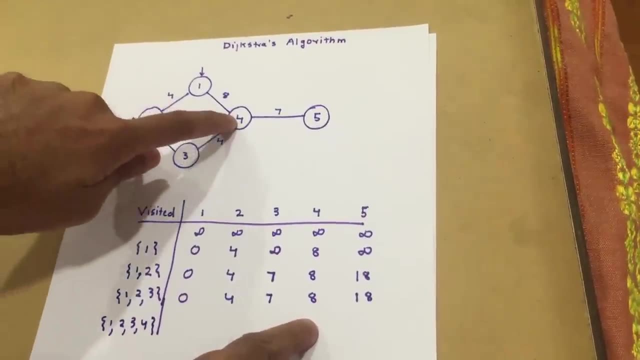 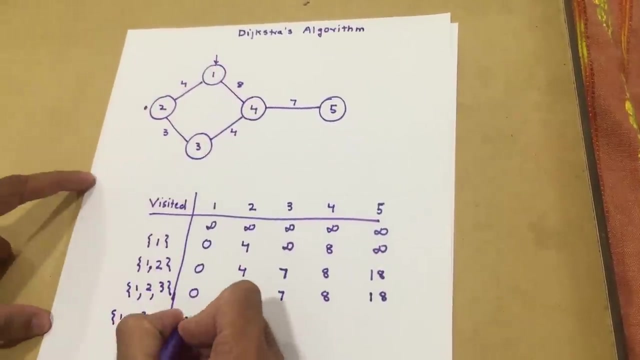 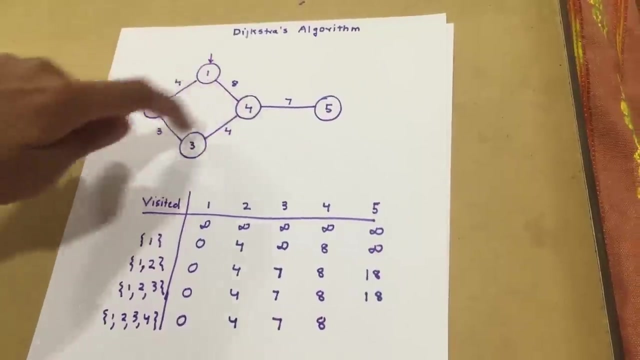 gonna visit node four. okay, so now we are on node four. so for node four, node four is connected to one and three. so first I am gonna write down these distances. as it is, so node four is connected to one, three and five, but one and three already visited, so we will look at the distance from five. 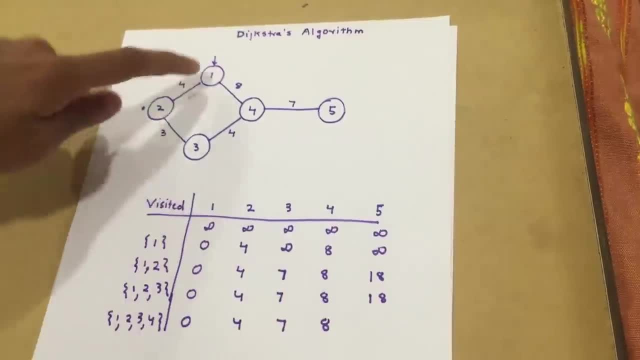 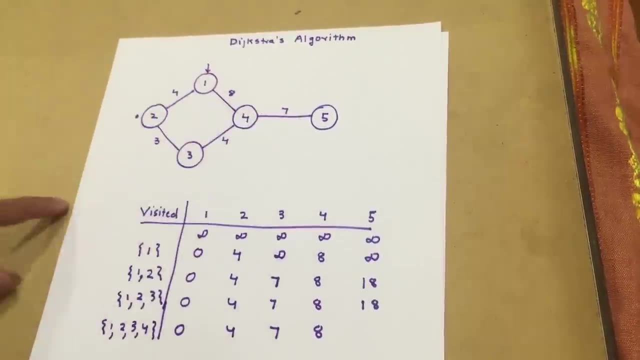 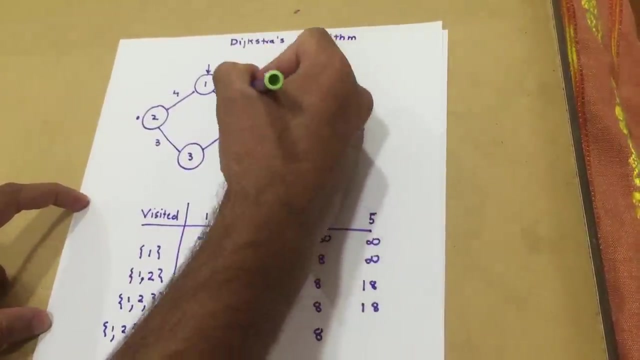 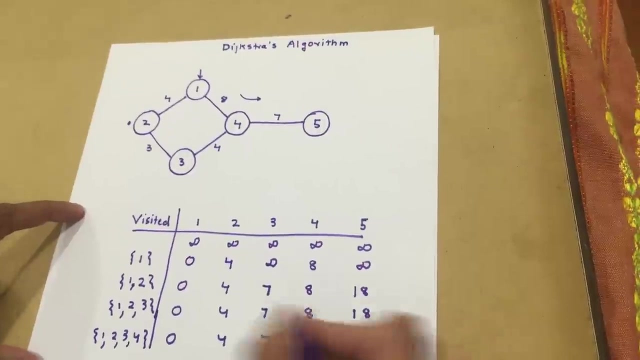 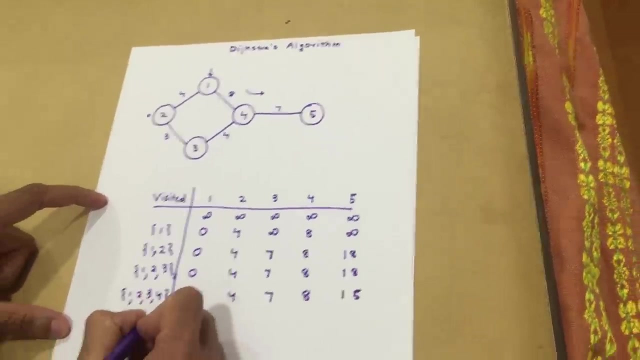 so initially the distance was eighteen. but now, if we go from the root node towards here, distance will be what? eight plus seven, fifteen, right? so initially it was eighteen. now the distance is coming to be fifteen. so we have to choose the minimum distance, right? so this distance is fifteen. so now we go to the fifth one. our distances are gonna remain the same. 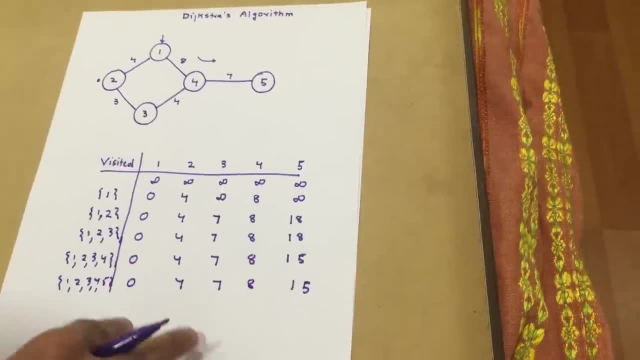 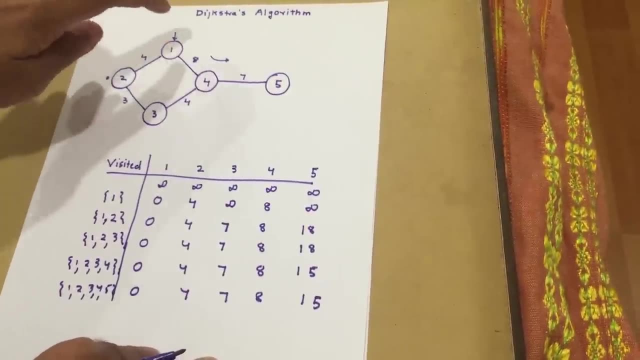 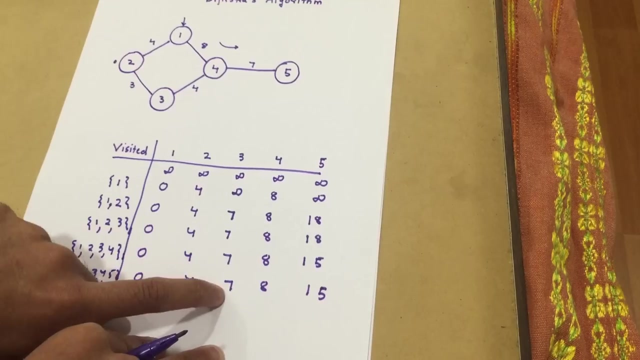 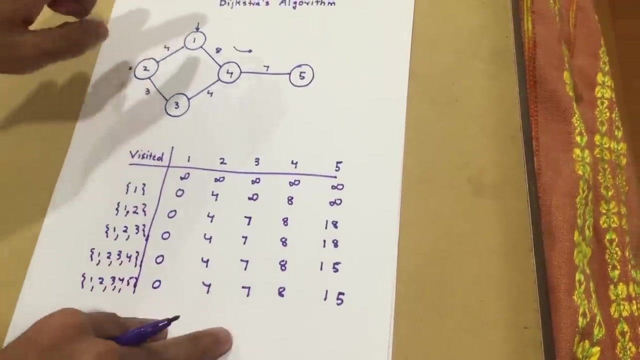 so basically, using this algorithm, we have found the minimum shortest distance of root node one with every other node. so basically, shortest distance of one from one is zero. the shortest distance from one to two is four, from one to three is seven, from one to four is eight and from one to five is fifteen. so if this is the root node, this is the sender. 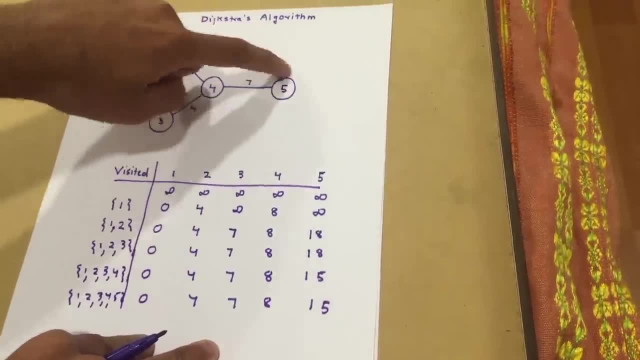 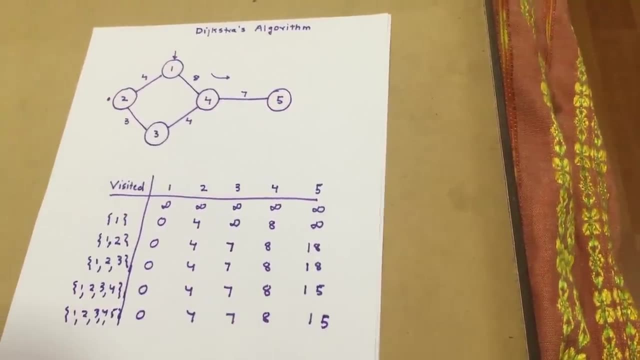 and it wants to send the message to the receiver. a router, for example, say at node five, then it will know that the shortest path is fifteen. so this is basically Dijkstra's algorithm. thank you guys.